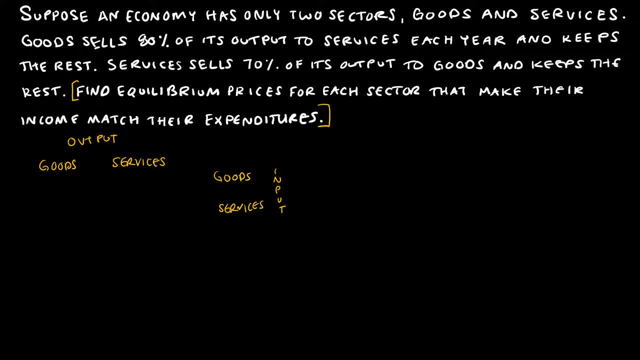 So, based on what we can read in the question, goods sells 80% of its output to services and keeps the rest- Again because I'm under output- And services sells 70% of its output to goods and keeps the rest. Now, how is this helping me? Because I'm going to make this now into an equation. 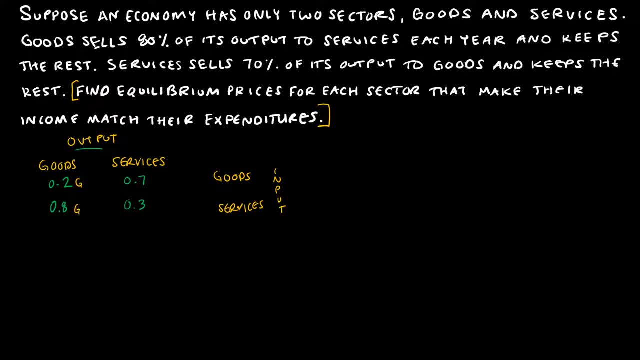 Little math magic. Let's use G for goods and S for services, And now take a look at what I have. I've got a system of equations. Now, what I notice about my system of equations is that I have a G on each side of the equation here, So I'm going to rewrite that guy into a new equation. 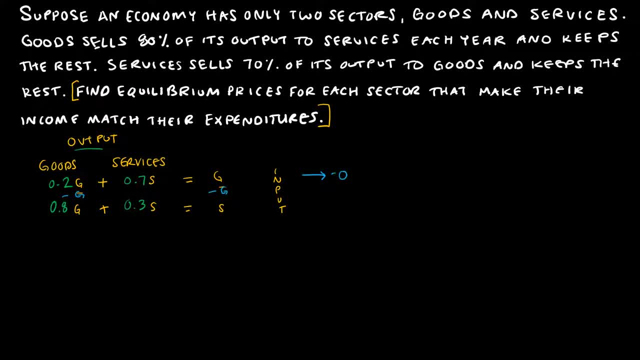 From each side, And that's going to give me negative 0.8 G plus 0.7 S equals zero. And then this one: I'm going to subtract S from each side, And that's going to give me positive 0.8 G minus 0.7 S is equal to zero. And I'm sure you've figured out now that this is just going to be written as an augmented matrix: negative 0.8 G plus 0.7 S is equal to zero. 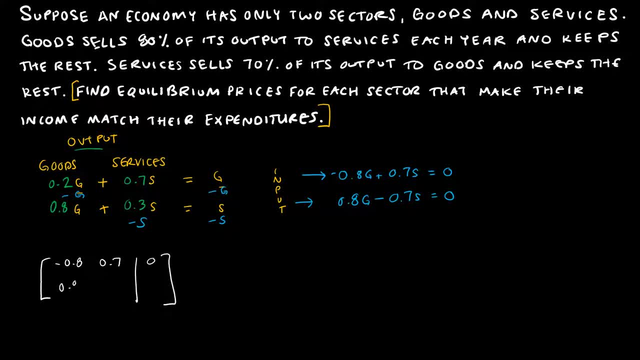 And then that leaps down to point zero. Positive 0.8, negative 0.7, zero, And doing a little bit of math and adding those two rows together to make a new row two, I end up with 0, 0, 0.. 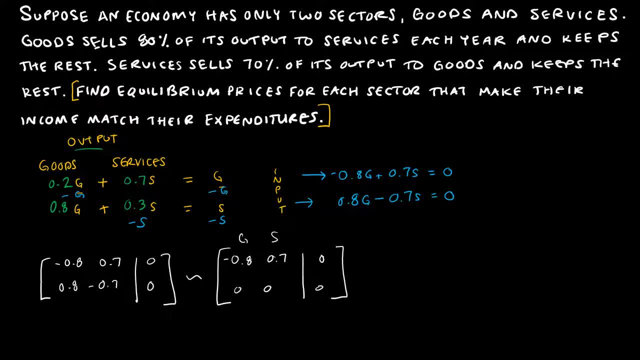 Which, of course, remember, this is my goods and this is my services, So that tells me that S is free. So, going one step further, because I don't like this, I'm just going to do another row operation to get my new row so that I don't have to deal with a negative .8, and that. 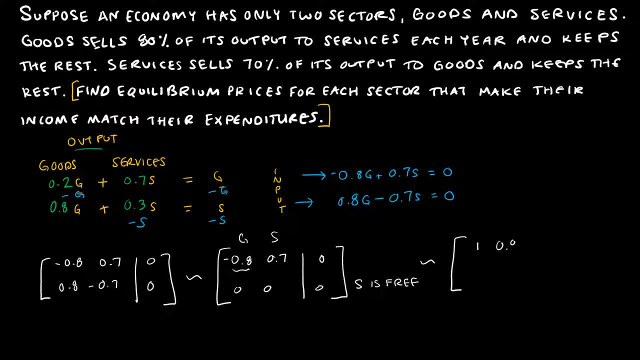 gives me one 0.875,- I'm sorry, negative 0.875,- zero and zero, zero, zero. So what does that tell me? Well, of course, that tells me, just as I did before. remember, I used to do x1,, x2,. 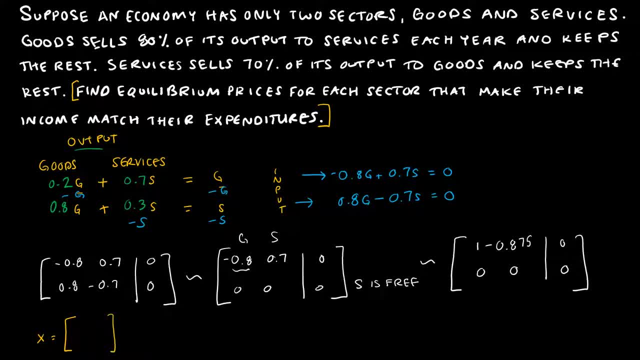 which is kind of what we're doing here. but now this is goods and services, And so this equation is 1g minus .875,. I keep forgetting that zero, I apologize. .875, s is equal to zero, And of course that means I'm going to write 1g as .875s. 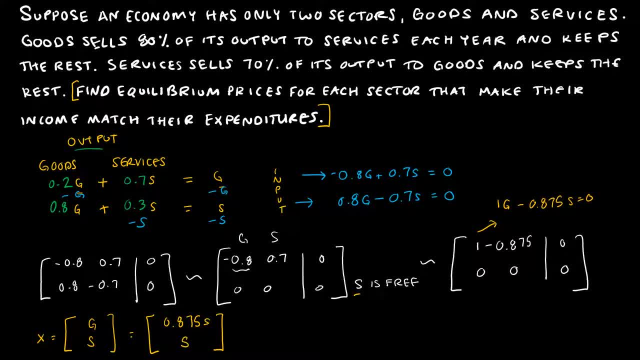 We already said that s is free, so that just makes s equal to s, And so if I'm looking for a solution here, remember I can just take the s out of this, and that gives me .875, one. So if I wanted to write that again in the parametric order, I would have to do the same. 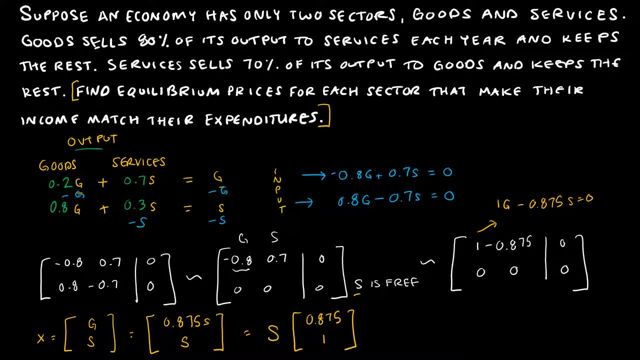 thing. If I wanted to write that again in the parametric form, that's exactly how I would write it. If I'm just looking for that general solution, remember my general solution is that g is equal to .875s. so when it says: find equilibrium prices for each sector that make their income. 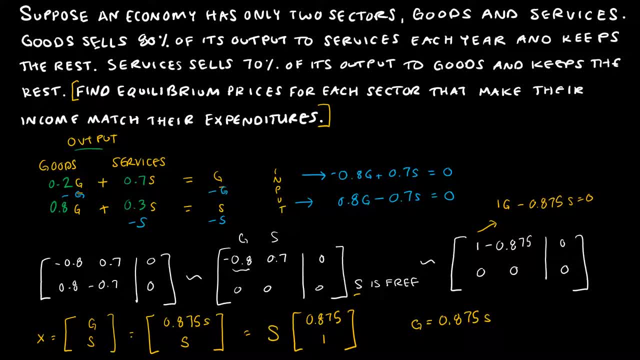 match their expenditures. really, what I'm going to do is make up some number for s and find out what g is based on that. So let's say that I'm going to let s equal 1,000, because that's a nice easy number. 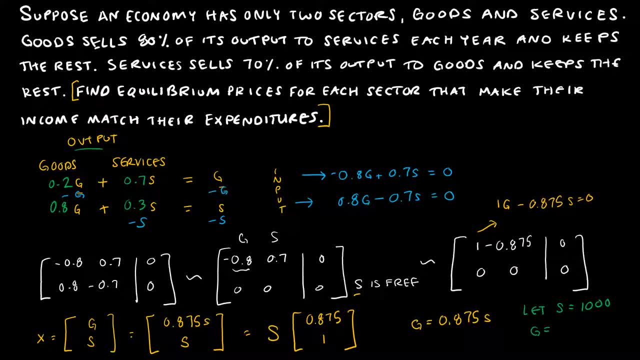 to deal with. then g would be .875.. And again, that's what the question asks: is: find an equilibrium price Now. does that mean that's the only correct answer? Of course not, because I made up s out of nowhere. 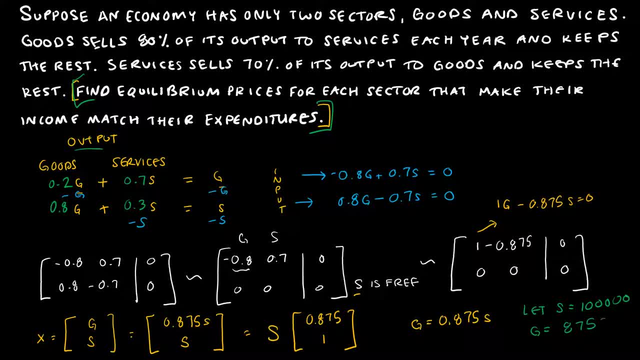 So let's say s was 100,000 instead. Well, that's going to change. Well, that's going to change g to 87,500.. So we can see that really, what we're looking at is the ratio of expenditures and output. from each sector.